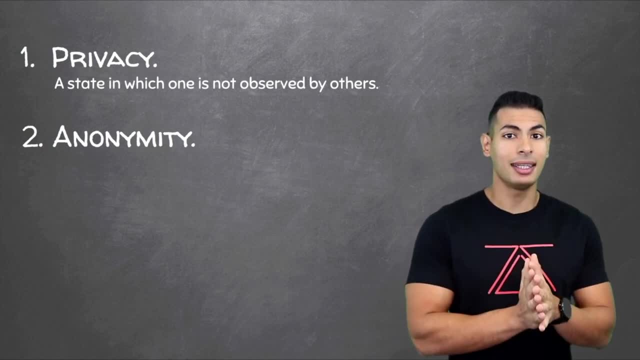 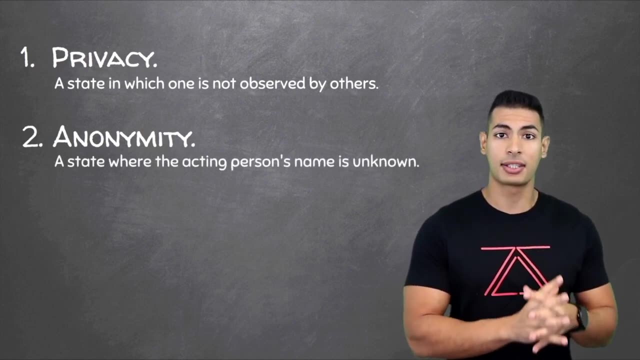 Anonymity, on the other hand, means that people can see what you're doing, but they don't know who you are. For example, let's say, while you're inside your house, you put a mask on and then you leave the house and start washing your car. Now people can see that there is somebody washing the. 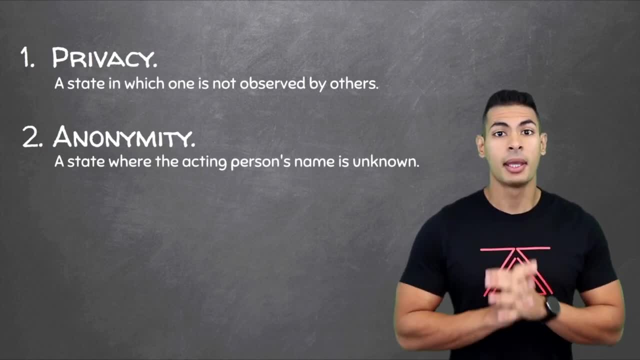 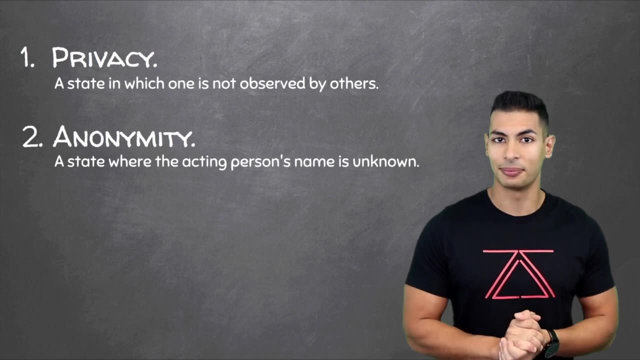 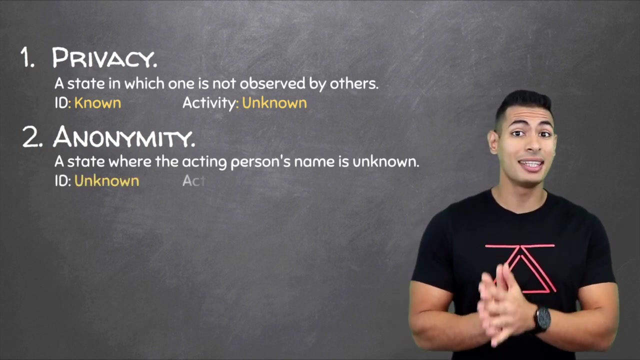 car so they can see what you're doing, They can see the activity, but they don't know who is that person washing the car because you have a mask. Therefore, you're hiding your identity. So when you're private, people know who you are, but they don't see what you do When you're anonymous. 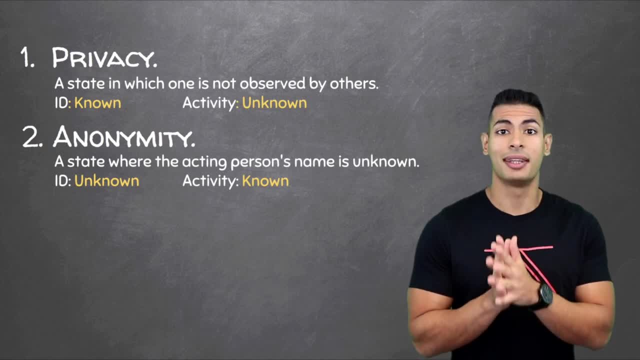 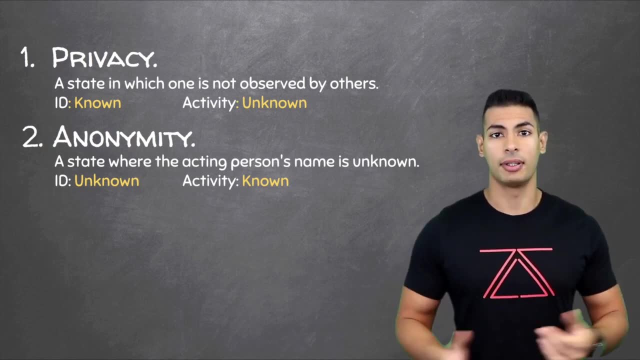 people see what you do but don't know who is that person doing that activity, so they don't know your identity. Now, on the internet, usually we just want to be private, so we don't want other parties to be able to see the messages or the emails or whatever we do on the internet. 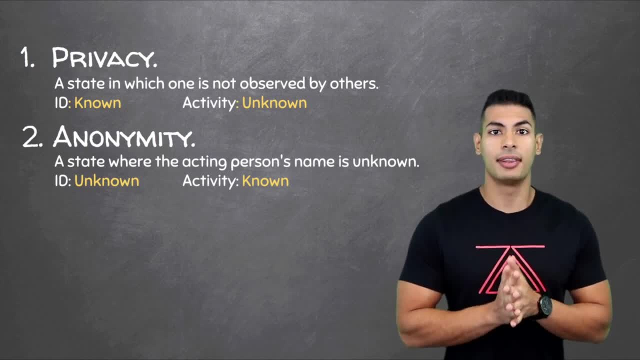 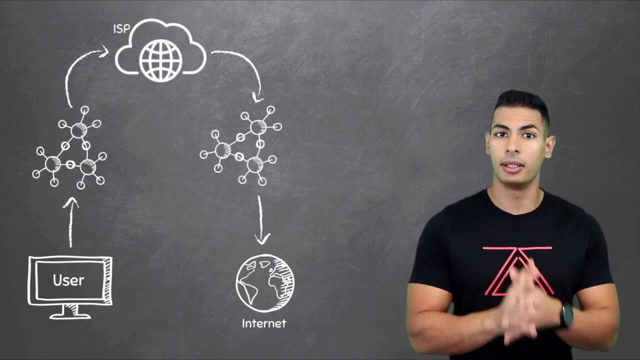 Unfortunately, though, it is very difficult to be private on the internet, because, in order to use the internet, you have to use resources that are not owned by you, So you have to use an internet service provider, and when you're accessing websites or using 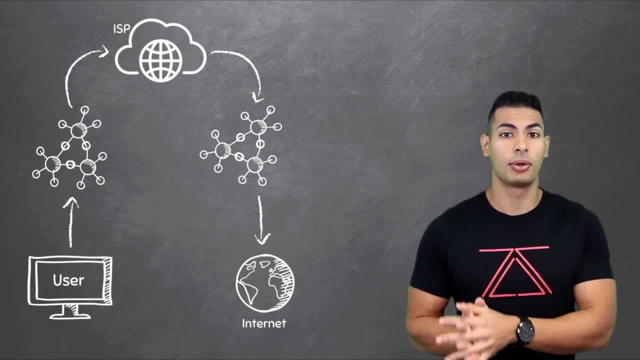 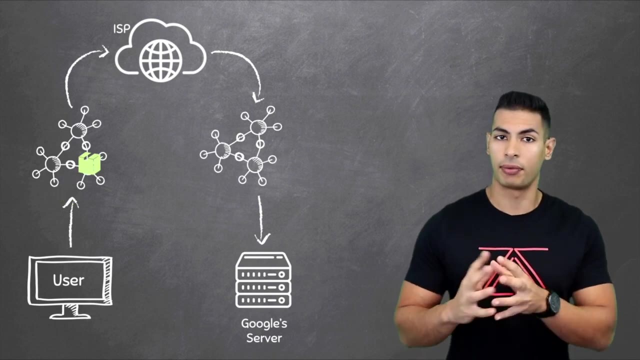 services. you're using servers owned by these services or by third parties. Therefore, you can't really control how your data is being handled. For example, let's say you try to go to googlecom. This request will first of all pass through a number of stops or a number of routers. 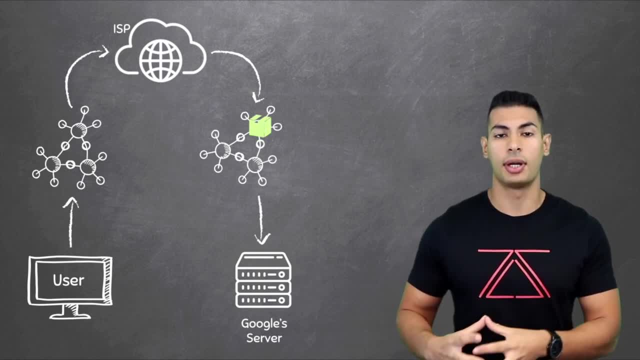 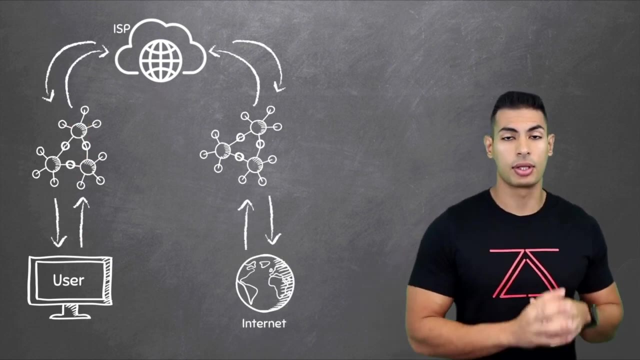 it'll go to your internet service provider, It'll pass through a number of routers and eventually reaches Google servers, which again are not controlled by you, And then you get your response through a similar route. Therefore, both your request and the response will pass through a number of stops that you don't own or don't control Anybody operating. 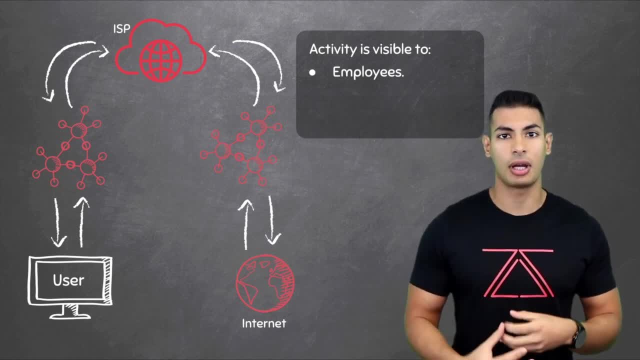 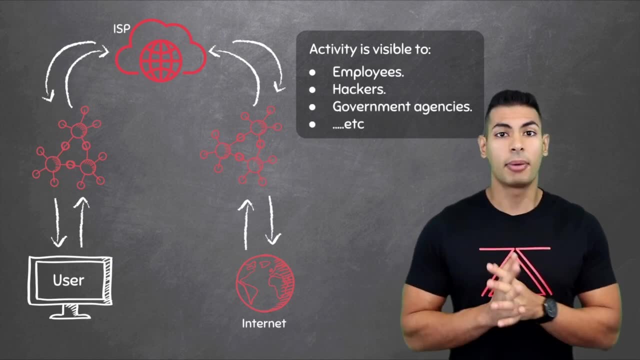 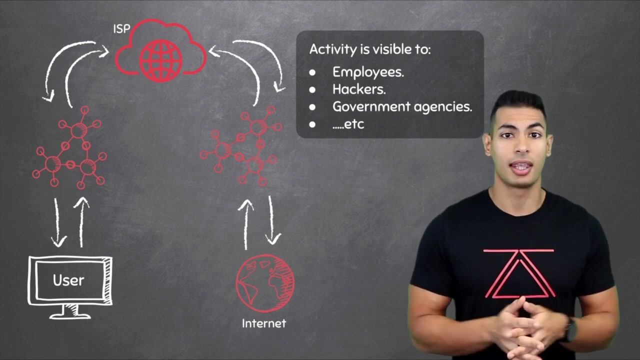 or working on these stops will be able to see your traffic. you will be able to see your activity. that but hackers and government agencies and other entities can possibly intercept these requests and responses at any point and therefore see what you're doing. therefore, your privacy is gone. 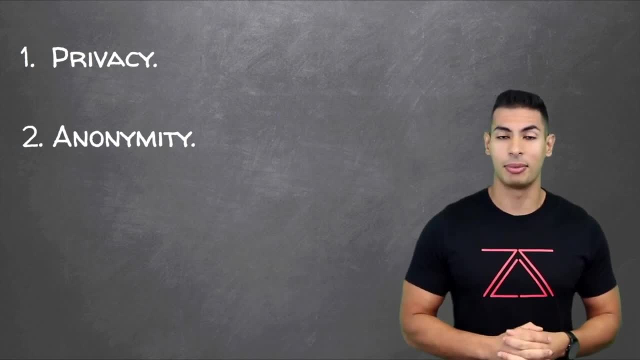 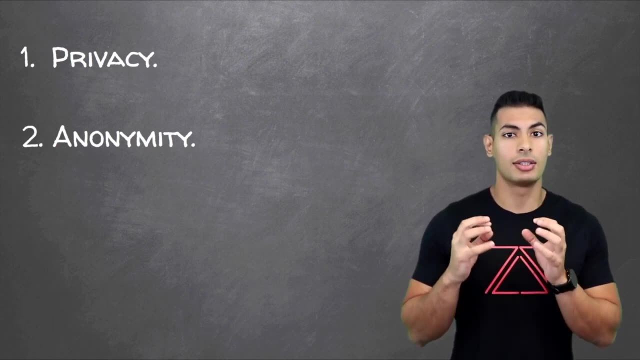 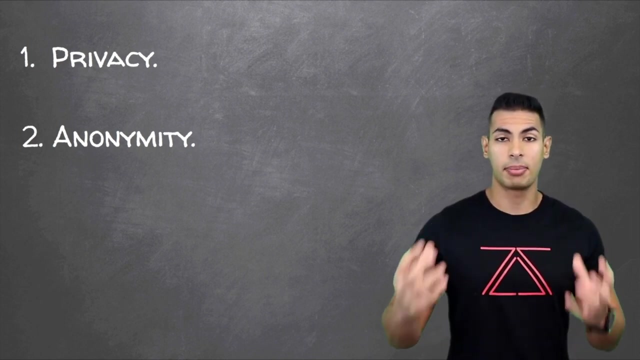 so we use encryption whenever possible in order to improve our privacy. but, like i said, there will be some points and some situations where it is just not possible to be private. therefore, the best solution is to try to become as anonymous as possible. so if anybody manages to intercept, 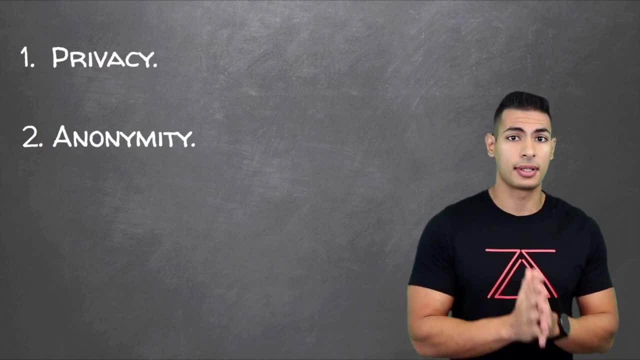 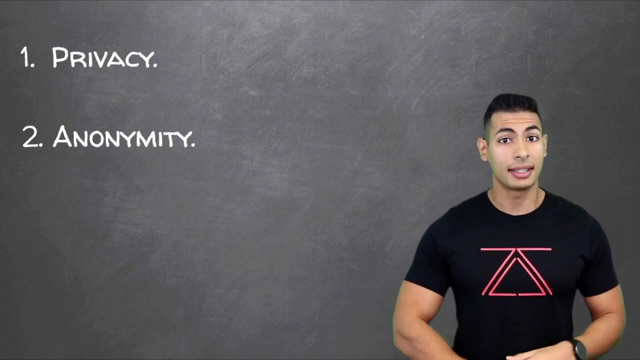 our data. they won't be able to link it to ourselves or to our identity. now there are some situations where people actually want to be just anonymous. for example, journalists usually prefer to publish sensitive posts anonymously so that everybody can see the post. so it's not hidden, it's not private. 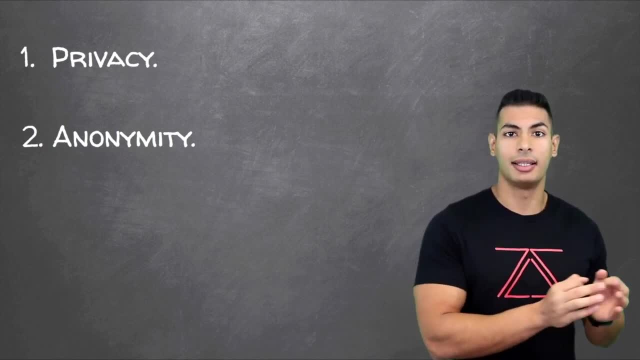 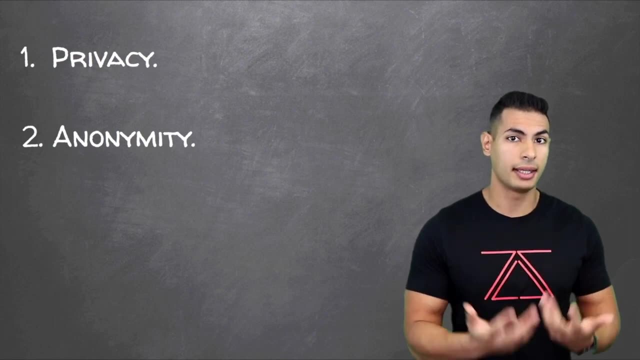 but at the same time it can't be linked- you can't see the posts, so it's not hidden, it's not private- to their real identity. this way the post will be linked to some kind of identity. so it will be linked to a fake name or simply just numbers or a ghost profile, but it is linked to some kind of 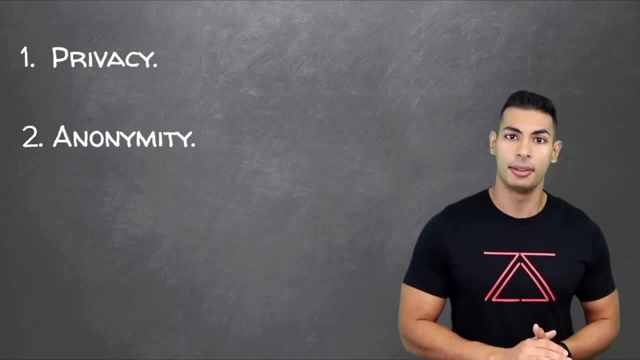 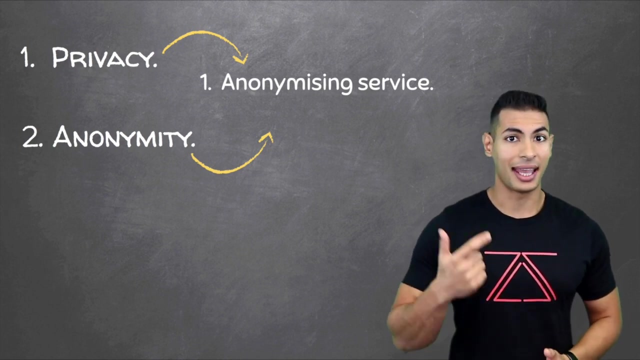 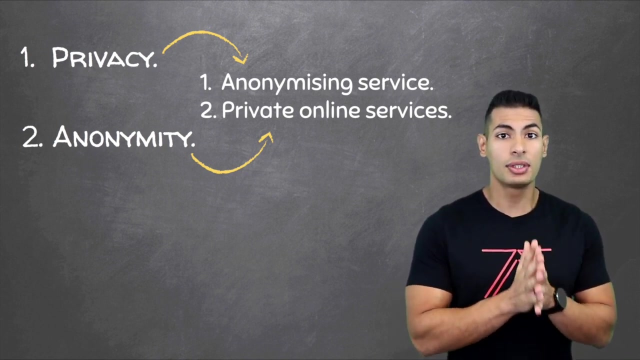 identity. therefore, this is known as pseudo anonymity. now, in order to achieve the above two things- to become more private and more anonymous- we're gonna need two things: first, we're gonna need an anonymizing service that will allow us to become more anonymous, and, two, we're gonna need to change our habits when it comes to using online services and use. 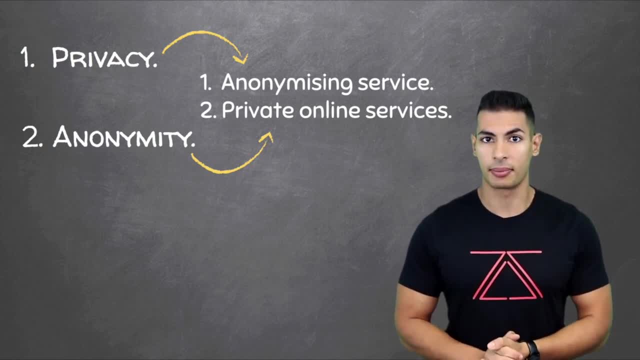 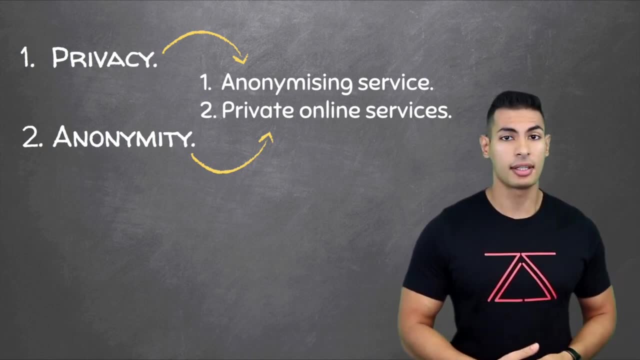 different services that are more private and more anonymous, because the search engines that you're used to, for example, google and bing, the emails that you're used to- gmail and the others- and all of the other services that you're used to use- are simply not private and not anonymous. they profile. 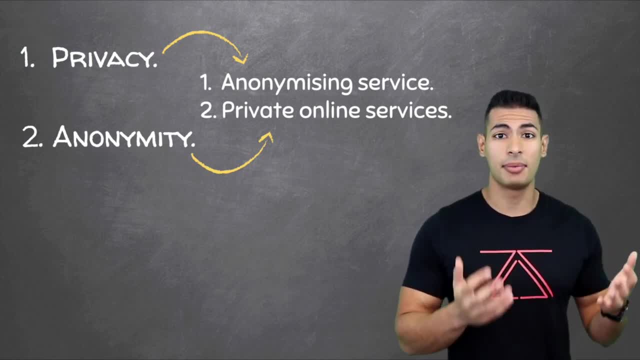 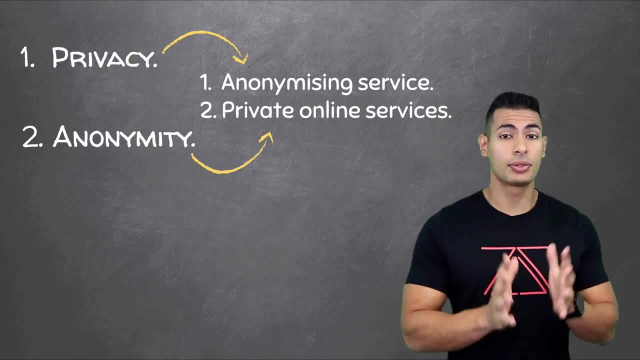 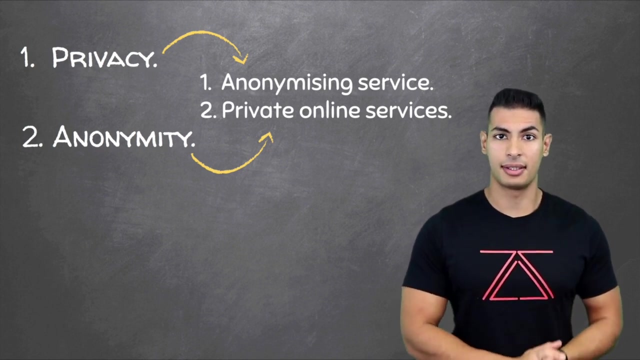 you, they collect data about you and sometimes even sell it to third parties. unfortunately, on the clearnet, there aren't a lot of useful online services that are private and anonymous. luckily, though, the anonymizing services that we're going to use from point one in order to 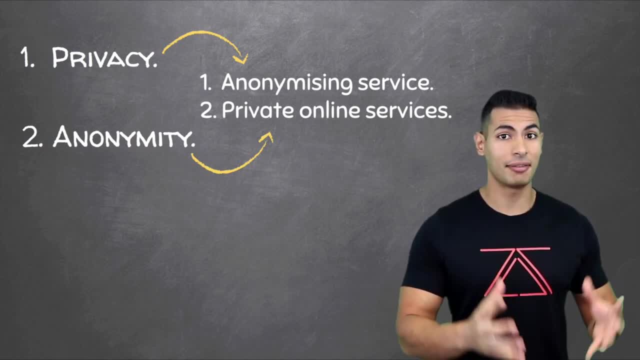 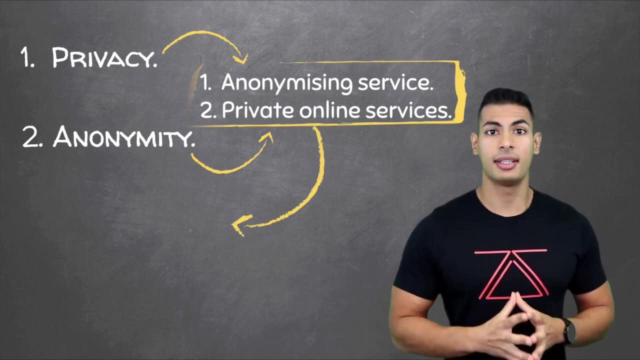 become more anonymous, also contain a number of services and websites that only exist within this anonymizing service or network. therefore, these are referred to as darknet or dark web websites or services. so we're going to need to change our habits and we're going to need to change our